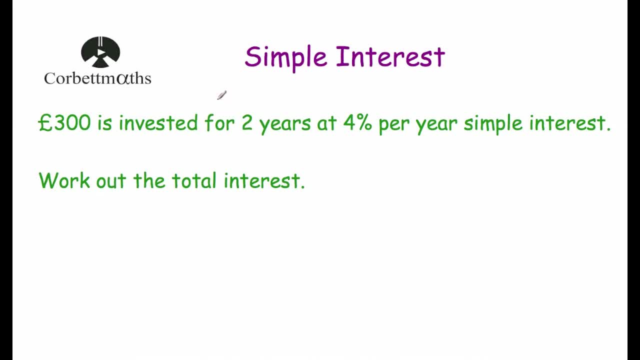 situations where it involves loans being paid back and things like that. So simple interest is where the same amount of interest is added every single year. So here we've got our first question. So our first question says: £300 is invested for two years at 4% interest, or. 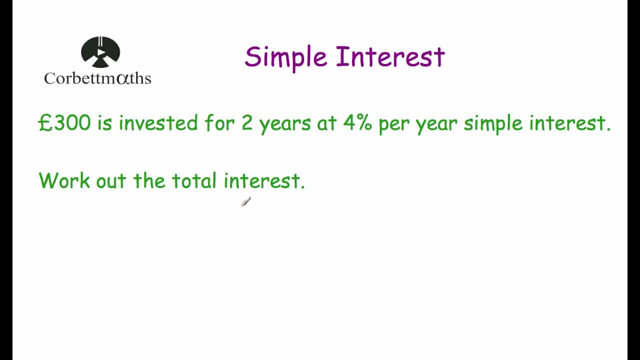 4% per year simple interest. Work out the total interest. So first of all, we know that £300 being invested, and for two years at 4% 4% per year simple interest. So what we know is that 4% of £300 will be paid for both. 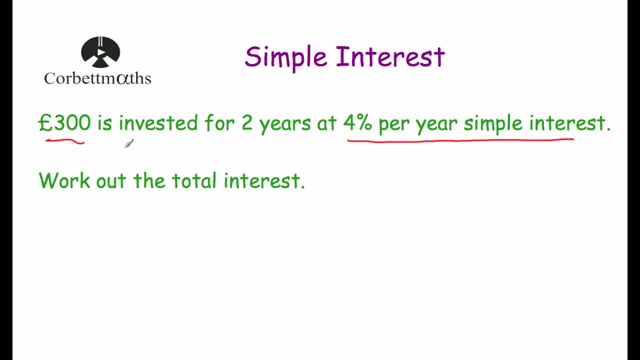 of those years that that money is invested. So first of all we need to work out what 4% of £300 is. So let's work out what 1% is- 1% of £300.. So to find 1%, we divide. 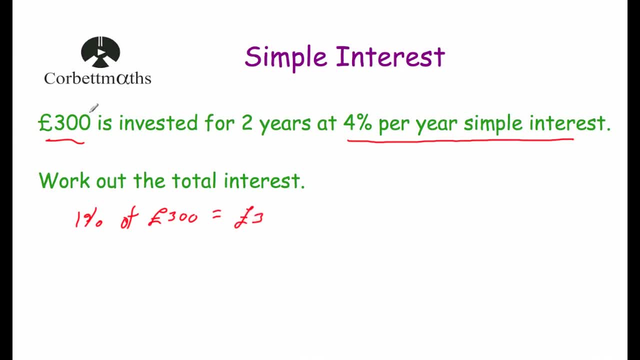 by 100 and that would be £3.. So that means that 1% of £300 is £3. and to find what 4% of £300 would be £300.. £300.. We just times that by 4.. So 3 times 4 is £12.. So that means that, because this is a simple 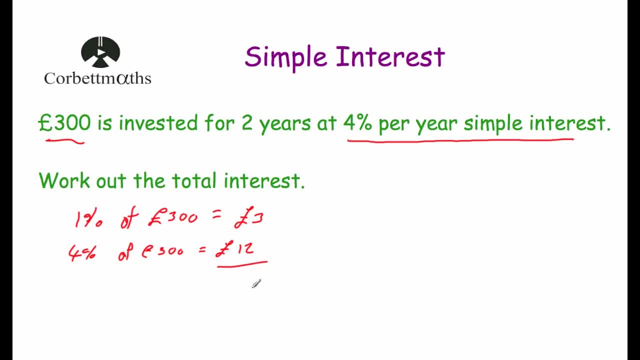 interest savings account. we know that £12 is going to be paid every single year, So we know it's invested for two years. So we're going to do 12 times by 2 and that would give us £24.. So that means that if this £300 was invested for two years at 4% simple interest, 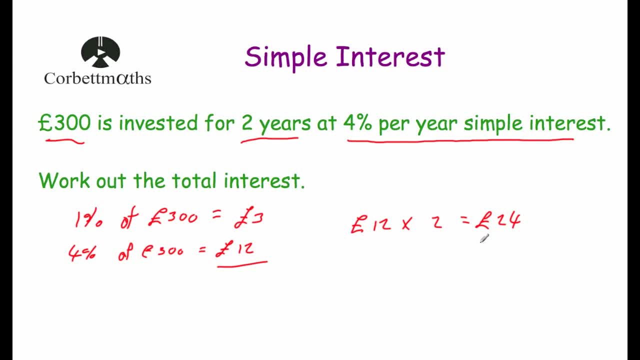 the total interest, the total amount the bank would pay the person who invested, it would be £24 and that's it. If the question was worded slightly differently and instead of it asking what worked out the total interest, and it said how much money would there be at the end of the two years? 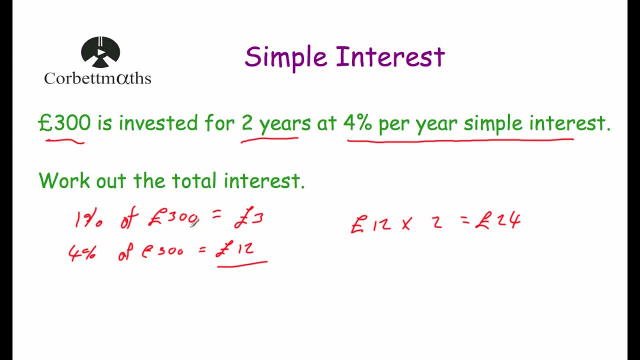 we would add the £24 onto the £300 and say the answer would be £324 for the total amount that would be. that would be how much money there would be at the end of the two years. But the question just were asked: you for the total interest, and that would be £24.. 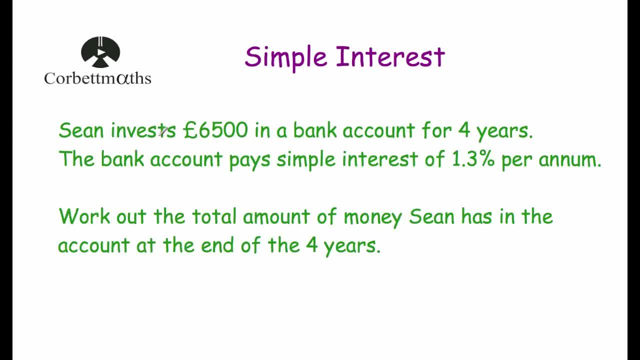 Okay, let's have a look at our next question. So next question says: Sean invest £6500 in bank account for four years and the bank account pays simple interest. it's very important that you see that simple interest of 1.3 percent per annum. per annum is another term for per year, it just